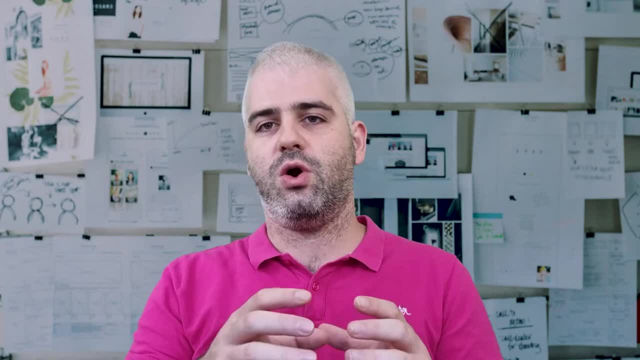 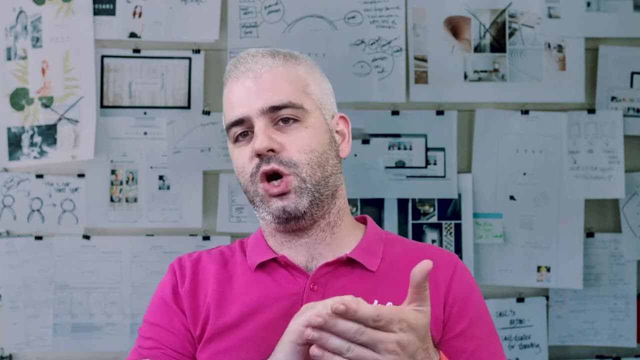 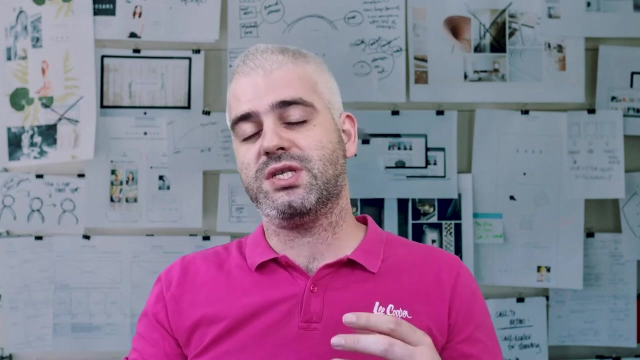 do is we would have like a process or the customer lifetime journey and we'll have like key points in it and analyze customer satisfaction at all. those key points identify where we lack something and figure out ways to improve it. The best part about those customer satisfaction questions is that they're really easy to ask. They take but a second to answer and they don't require the customers to perform something complex. It's pretty simple. We just need to find the right spots to ask those questions and not do that only after let's say we release new features, because everyone loves new features. 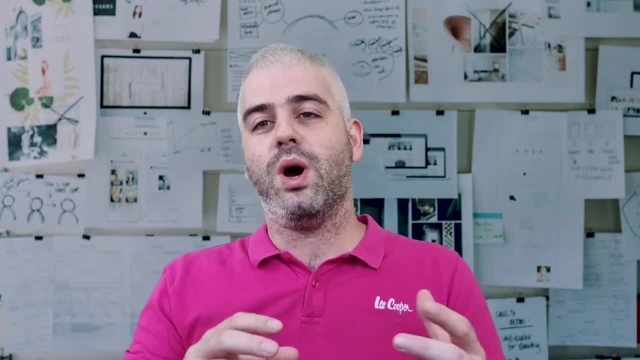 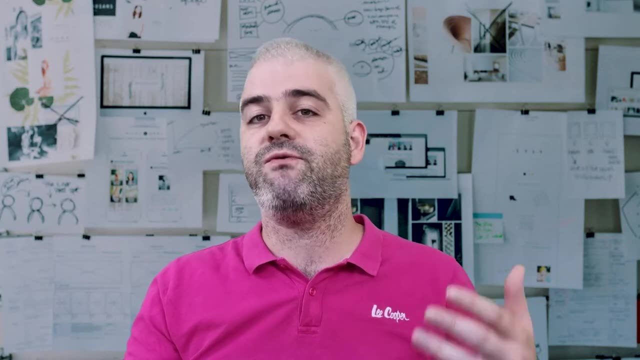 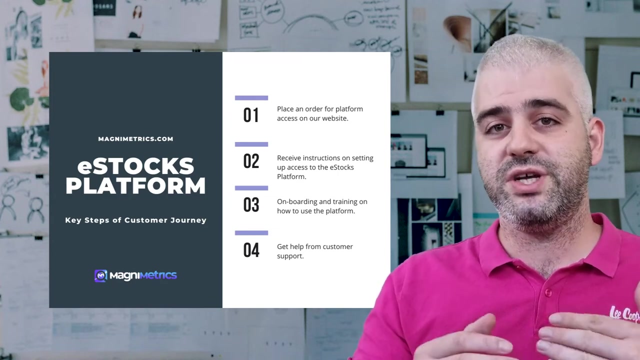 So our score will be quite skewed upward Once we identify those and for the purpose of this video, let's look at the basic like lifecycle journey with four steps. The first one is the customer visits our website and orders access to our platform. They then receive, in the second step, instructions on how to log in, enter their credentials. 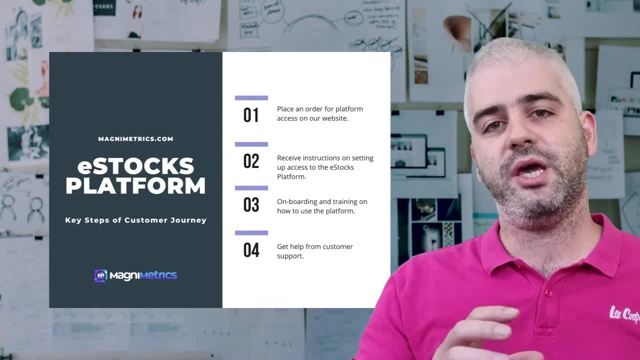 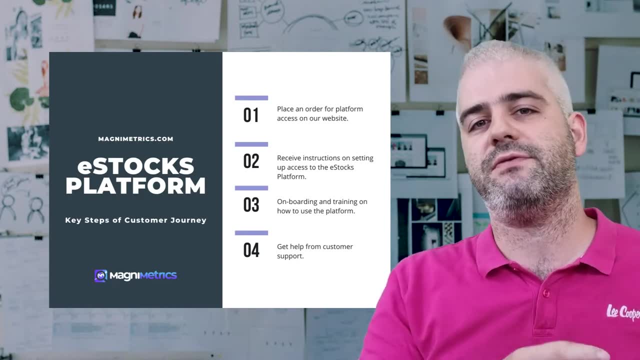 and set up their whole profile. The third step would be them completing the onboarding process, like watching tutorials, maybe reaching out to a customer- They also need to be a customer support representative and things like that- so getting them ready to use our product. 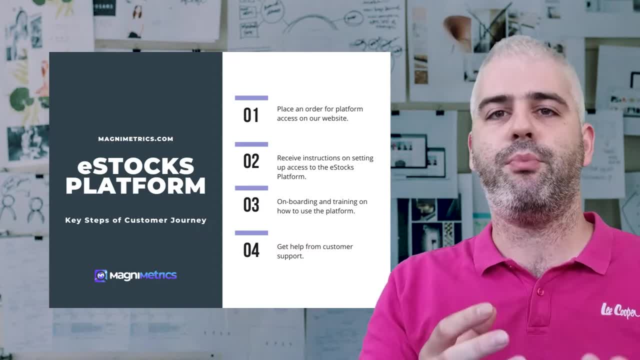 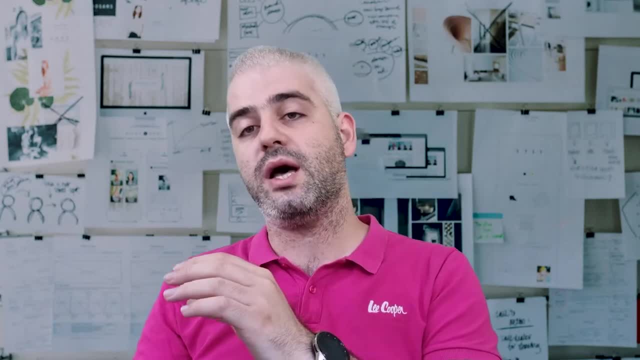 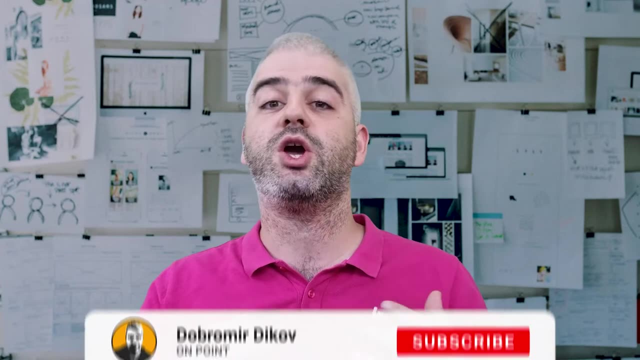 And a fourth step might be- any time they need customer support- how this was handled. Now that we have those four steps, we'd ask how satisfied our customer was with the process after each of those four steps And once we have this data for a bunch of customers, we can go ahead open Excel and see how easy 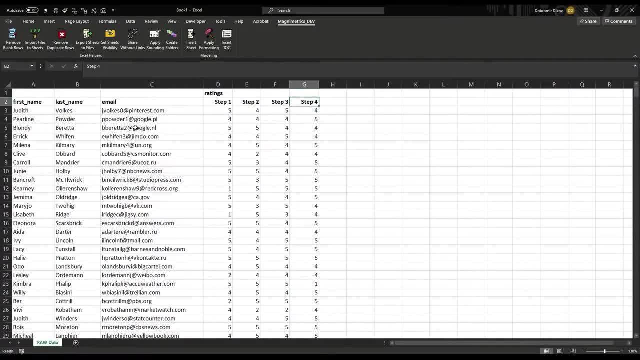 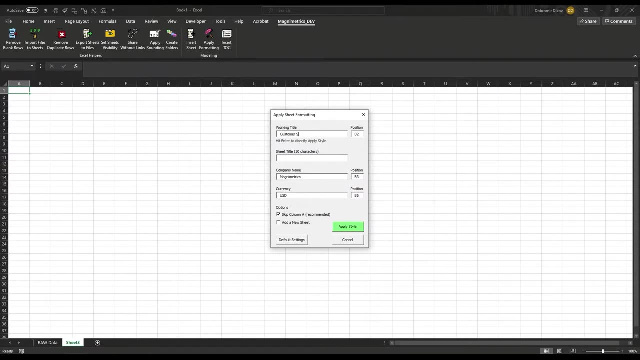 it is to analyze customer satisfaction. Here's the raw data that I have. So I have our customers and their ratings during four steps of their customer journey. So when I add a new sheet and apply some formatting to it and it's going to be my customer satisfaction. 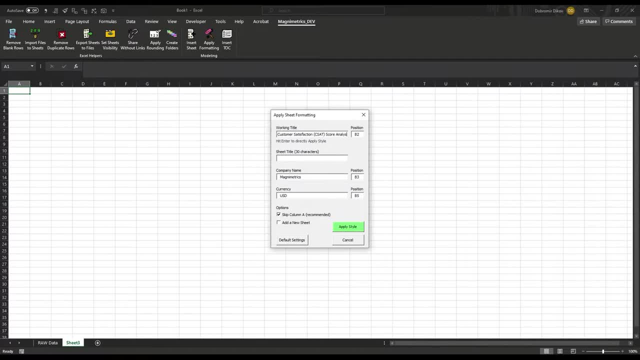 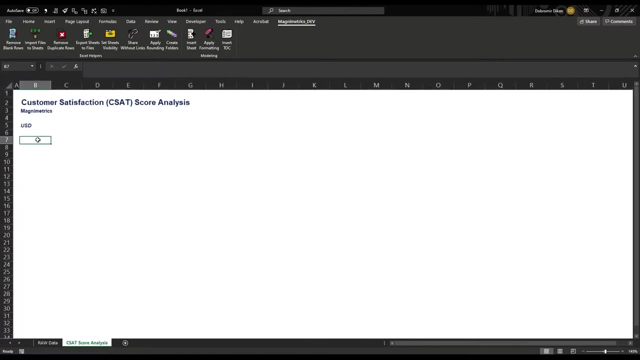 or CSAT score analysis. is that score analysis for the sheet title? Okay, let me zoom that in a bit. What I want here is: at first, I want to have the step. it's going to be my step one all. 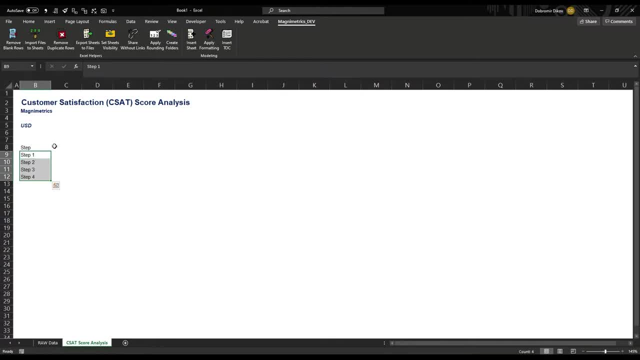 the way to step four, I also want to have the number of ratings, and this is going to be my number of ratings that I'm going to summarize here. So let me just format this accordingly, and then it will make a bit more sense. 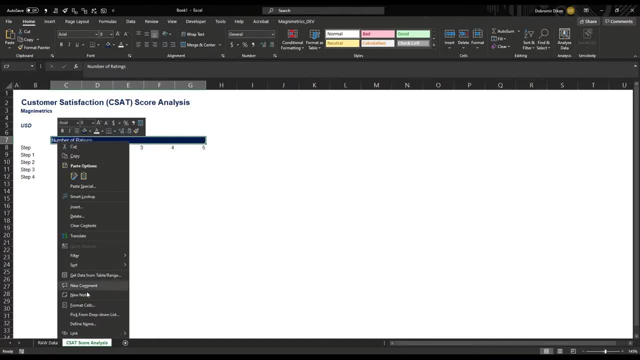 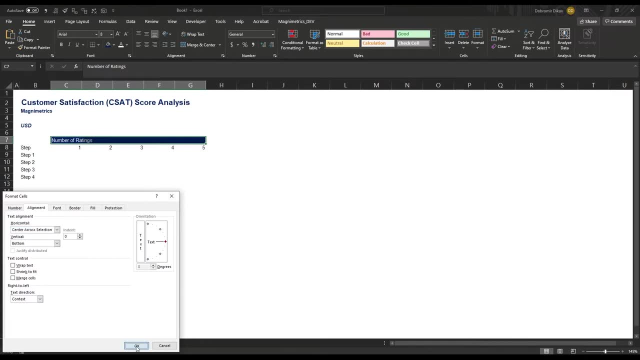 And here's a quick tip: instead of merging those, I'm going to do right click format, cells, alignment and horizontal center across selection. Okay, let's bold that. I want those bolded as well, And let's give them a nice. 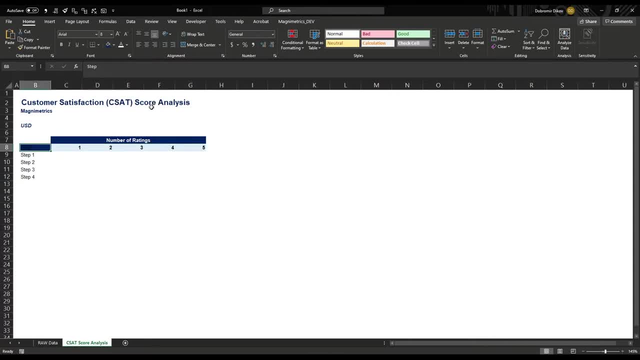 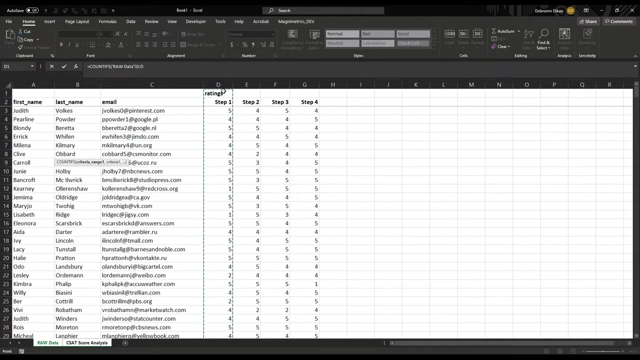 Okay, Okay, Okay, Okay, Okay, Okay, And this here will be our regular Okay. so here I want to get my numbers of different ratings. To do that, you're going to employ the count diffs formula. I'm going to go to my raw data and I'm going to count the first step where it's one. 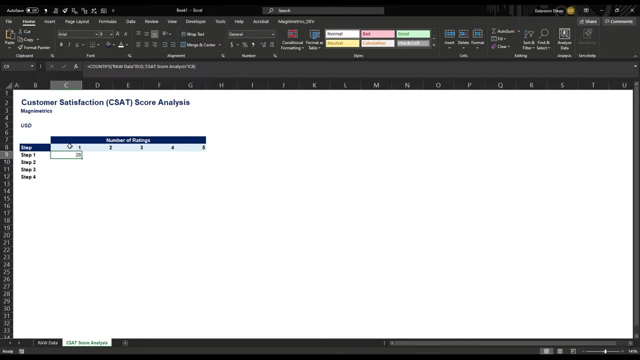 Okay, Okay. we have 28 people in our first step. that gave a rating of 1.. What we can do now is just fix that, because we want to be looking at the first step. So I'm going to press F4 on the D on this column here for step 1.. 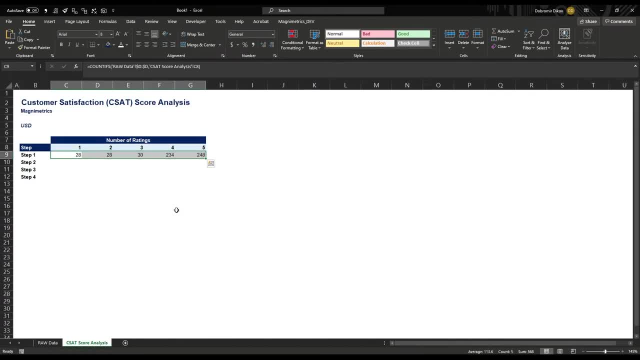 Now we can just expand this to the side and we have, at step 1, our survey that we did. we have a breakdown of different ratings that different people gave. So we had 28 people give it a 1 and we had 248 give it a 5.. 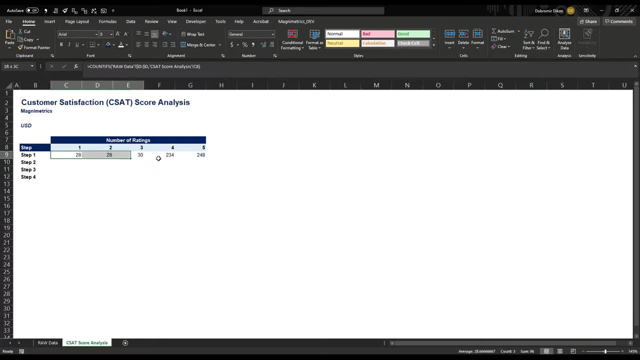 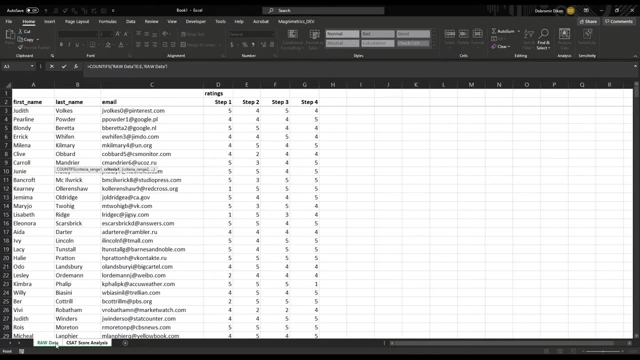 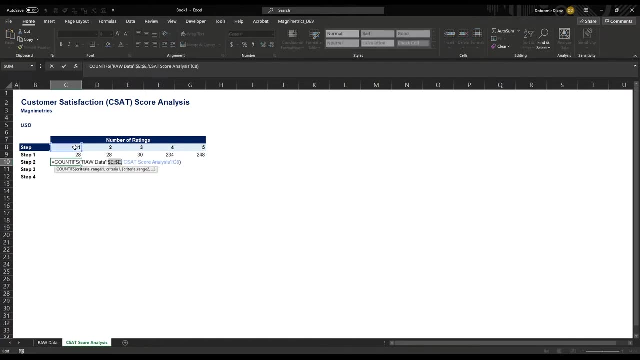 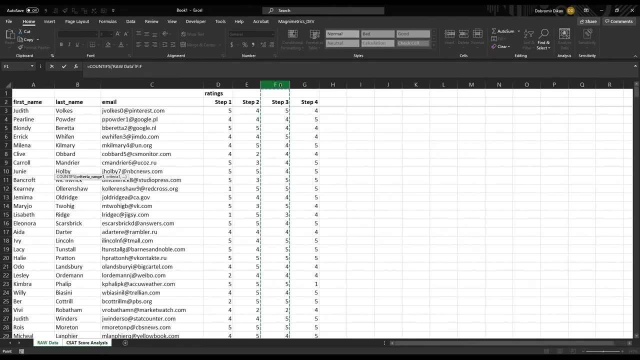 Let's do the same for the next batch: count divs. So step 2.. Okay, Comma, go back here, and I want it to be at 1, let's fix this one as well. count divs want to count column F for step 3, we're going to fix it right here, comma, and I want it. 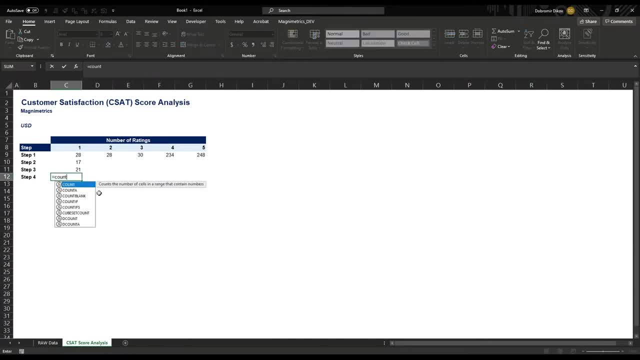 to be equal to my rating of 1 and count divs. my last step: We're going to submit it just here. Fix it as well, and I want it to be a criteria to be 1.. Okay, Now that we have those and we fixed the columns, we can just copy them to the side and that's. 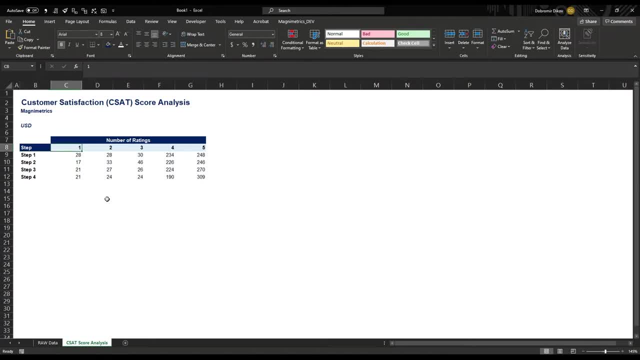 a summary of how many people gave each rating at each step. Now let's go ahead and calculate our average rating, and this is one of the ways to actually analyze customer satisfaction is to look at the average rating. I don't think it's the best idea, and I'm going to show you why. 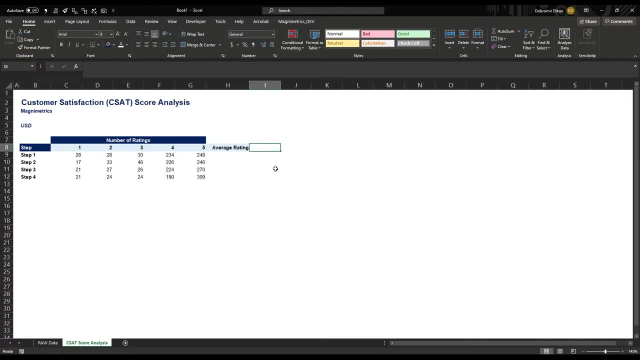 in just a second. So, apart from the average rating, of course, we're going to calculate our customer satisfaction score and outline why it's the better metric. If I can just copy this here, okay, and you see that it's already centered because it copies the. 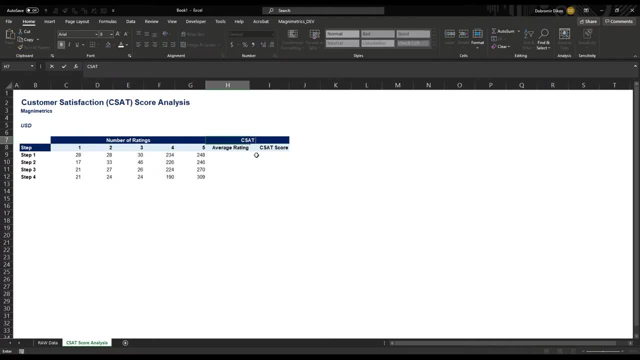 formatting. So this will be our customer satisfaction score calculation. Our average rating is pretty simple, So we just need the average, but weighted, because we have different people giving different ratings. So what we can do is use the sum product formula, And what we do with 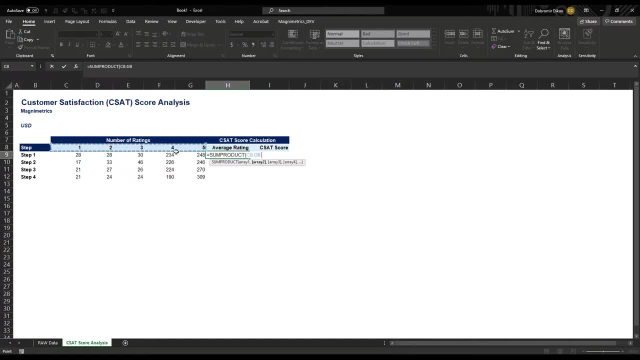 the sum product formula. you can just give it two areas and it's going to multiply each of the elements, So one times 28,, two times 28,, three times 30, and so on- and sum those. Then I want to divide this. 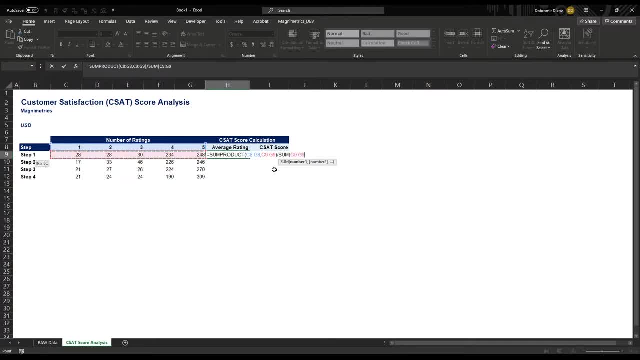 over the total number of ratings that we got, which is this here, the number of ratings given: Okay, 4.14, I think, yeah, Okay, let's make this formula easy to copy down. So if I can just fix those here, 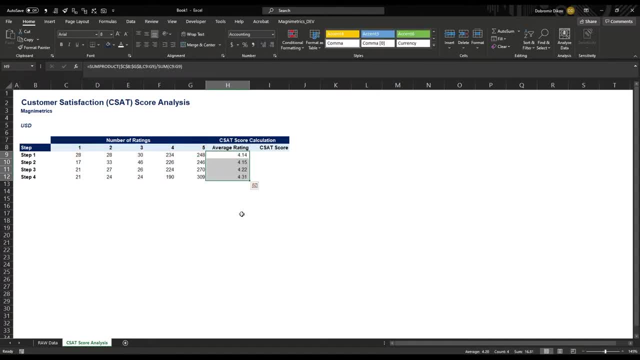 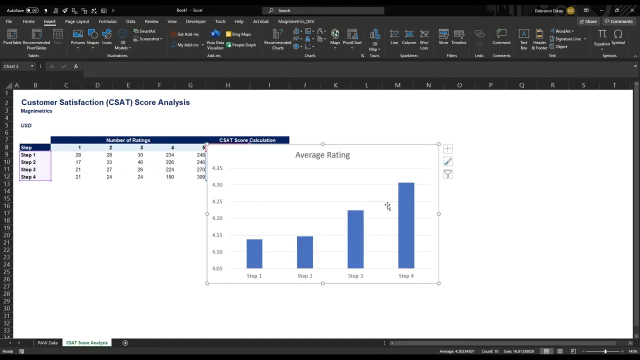 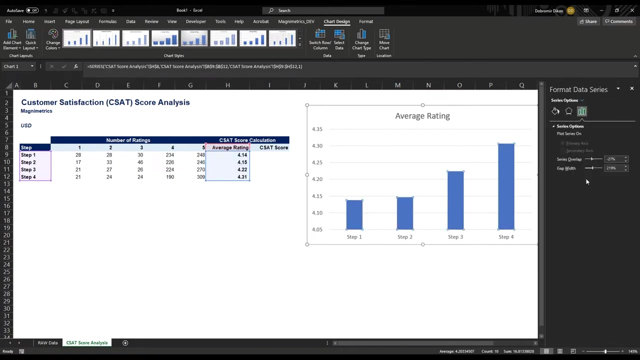 we can then copy the formula down with control D and get the average rating for each step of our customer journey. We can see that we're actually doing pretty good. Just grab those and add a chart to illustrate it. Okay, so here we have our average rating, step one through step four. Just format that a bit So. 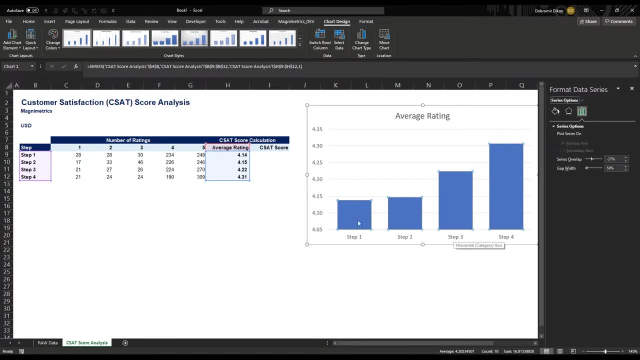 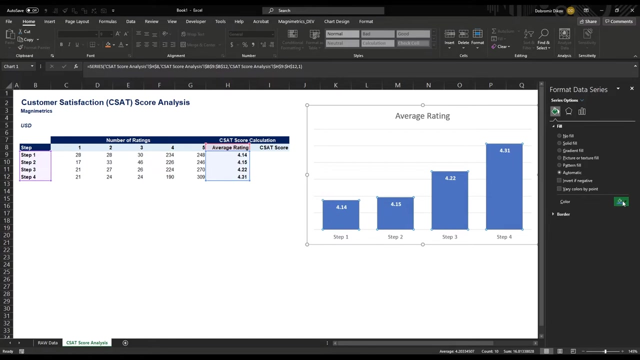 in that 50.. Let's get rid of this and just add data labels here, And I would like those to be on the inside end Control B to bold them And let's make them white. And also this thing here: let's make sure that it's consistent. 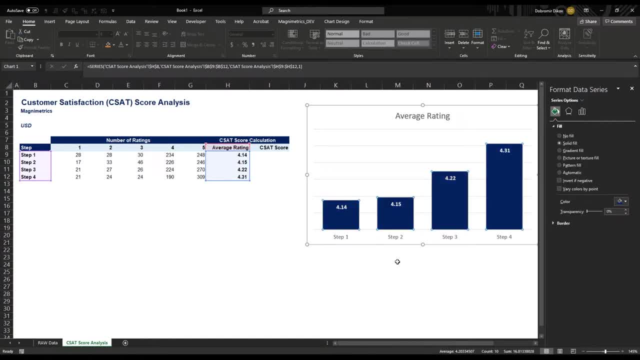 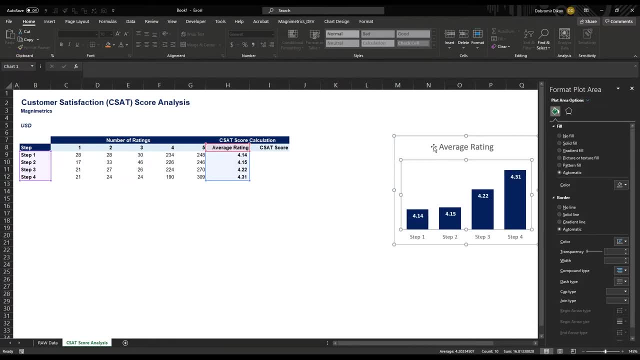 with our coloring. So let's make it our dark blue, And I don't think we even need those here. Okay, Okay, decrease the size of this a bit. So now we have a really concise chart showing us how we did at each step, And you can see that each step does a bit better. 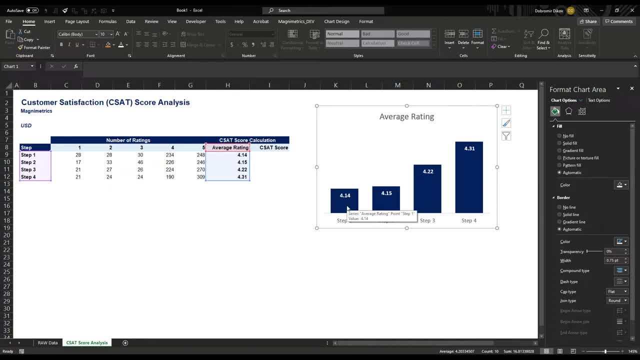 And this can very well be the case when at first they're still not sure if they're going to be a part of the longer journey. So they're not exactly fully aligned. But as we progress and we deliver to them, they're more and more satisfied. So let's see how this works. 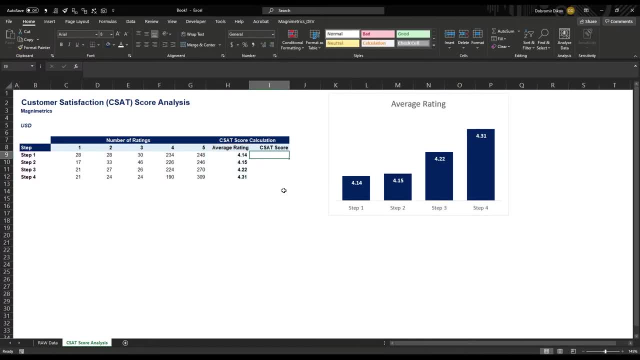 Okay, Okay. So what I want to do now is we're going to utilize this chart to try to calculate our customer score And, yes, This is the best case scenario. What happens if we decide to calculate our customer score? And remember, our customer score is pretty much the sum of our 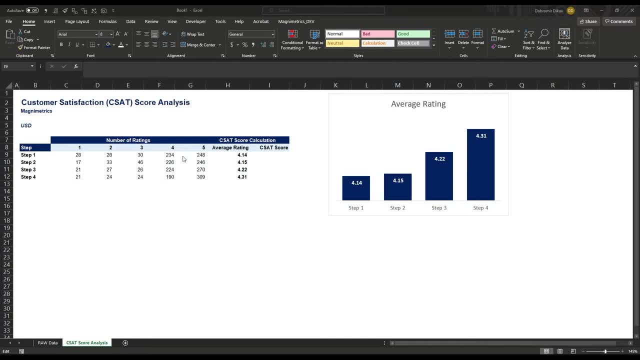 fours and fives- So those that are satisfied- divided by our total service. this will be the sum of our fours and fives- Yes, Divided over the sum of all weights. Yes, So those that are satisfied, divided by our total service. 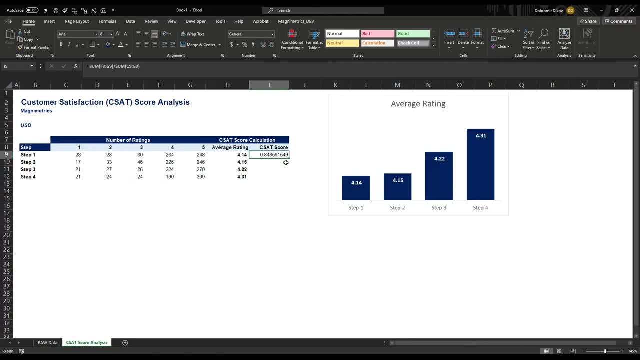 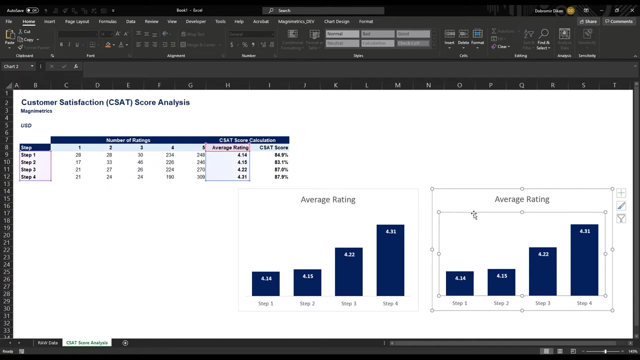 Our fours and fives. Okay, So those are satisfied. Okay, that we got. okay, let's copy that down, present it as a percentage. probably see something already, but the easiest way to actually illustrate this is to just copy this chart. okay, let's put those side by side and this here is gonna be our CSAT. 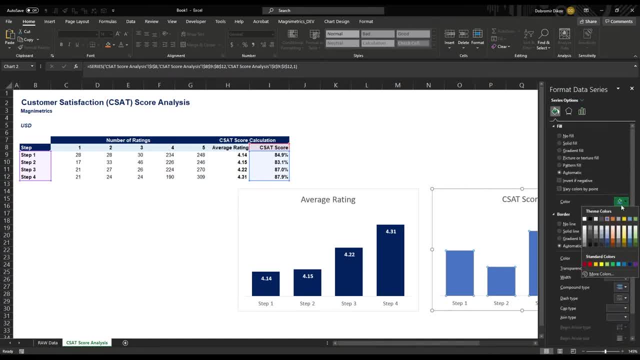 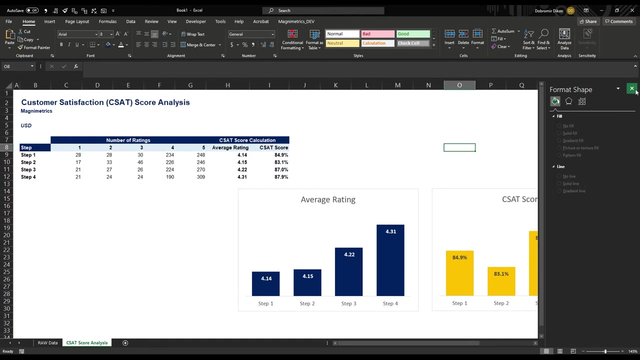 score and let me just make those gonna be consistent in our style and data labels. put them at the inside end and I'm actually gonna make those orange okay. so there's something that emerges immediately. so, even though our average rating grew, our customer satisfaction score actually dropped. it's not a huge drop, but it's still a drop that we need to. 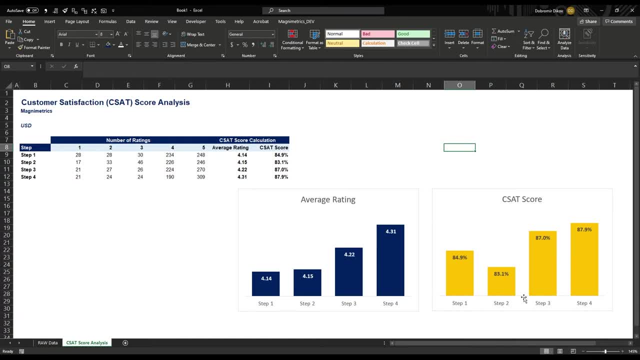 address. we definitely need to look into step 2, try to figure out why the satisfaction score dropped, and the reason for that is that the average increases because we have more people moving from 1 and 2 to 3. so you can see here we have 28 drop down to 17 and 28 increases a bit, but still and still, it's still a huge drop. 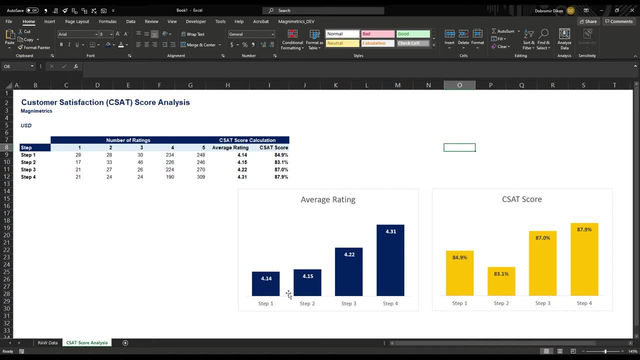 then 30 increases quite a lot. So this gives us a better average rating but at the same time the actual satisfaction score- the people that are overall satisfied- drops. That's pretty much how to analyze your customer satisfaction score, And you can extend that to have like 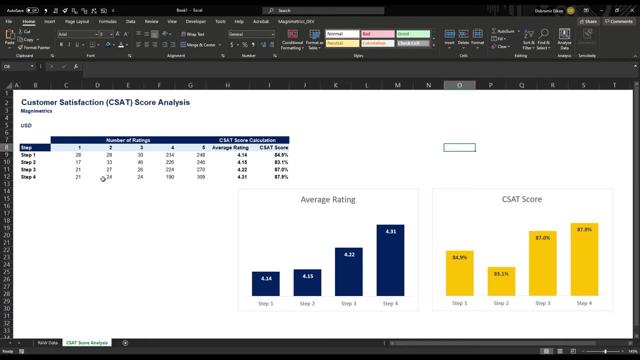 you can track each step over periods. So let's say, instead of having the steps here, we can be just looking at one step and having, like each next month, what it looks like, and then we'll be able to see the progress and figure out where we need to tweak our procedures. 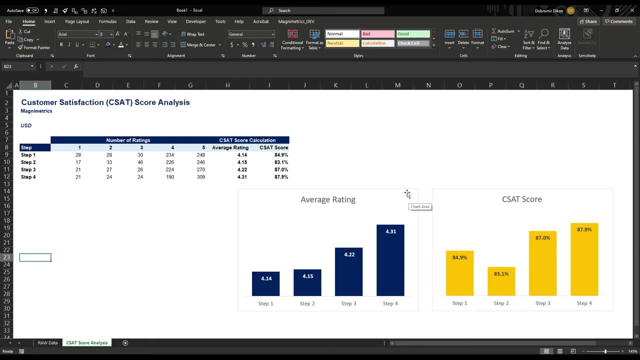 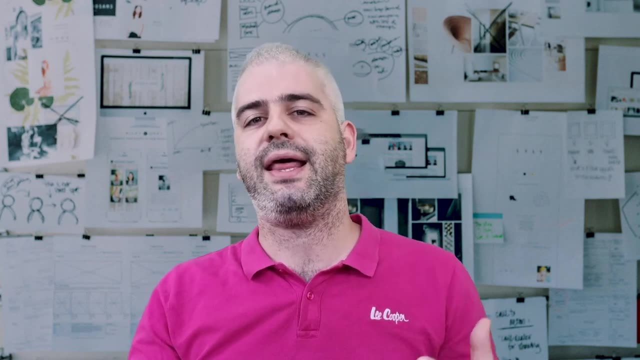 in order to ensure better customer journey, which would result in more satisfied customer base, which, of course, would increase retention and the bottom line. As you saw, it's really simple to just pull the data in Excel and analyze it And, by inputting the data. 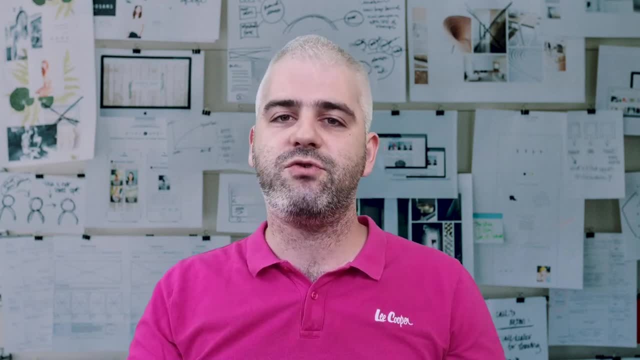 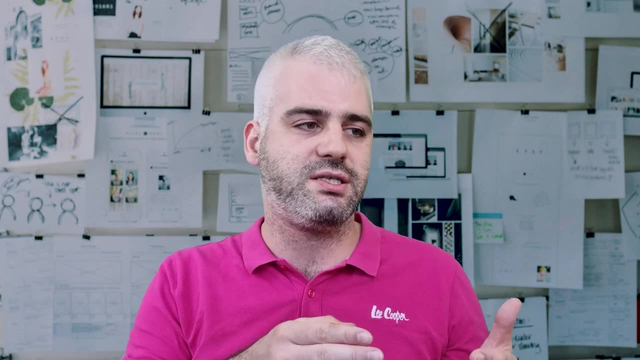 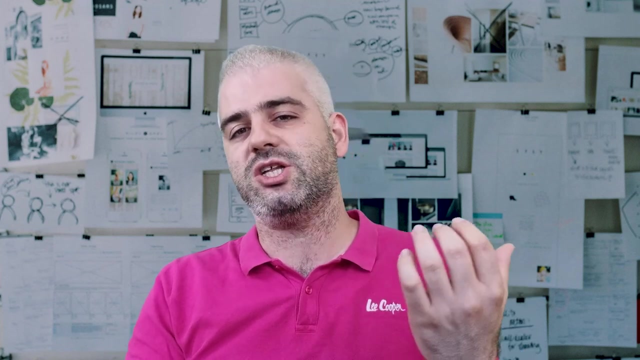 by implementing the customer satisfaction score and not only looking at average ratings, you can actually see that we might uncover interesting insights. In our current scenario, you notice that while our average ratings were growing, our customer satisfaction score actually dropped at our second step. 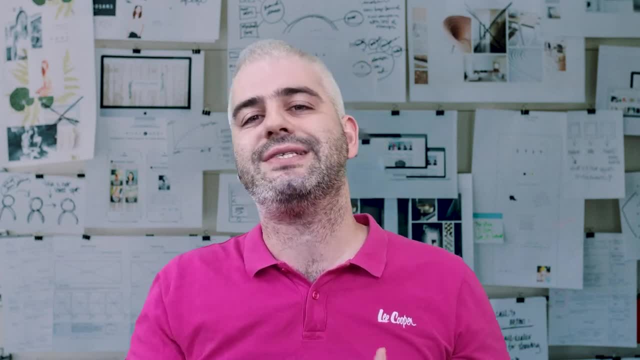 So what we usually do next is review the process for this second step, talk to the people that are involved in it and try to figure out what results in in the next step. So what we usually do next is review the process for this second step.